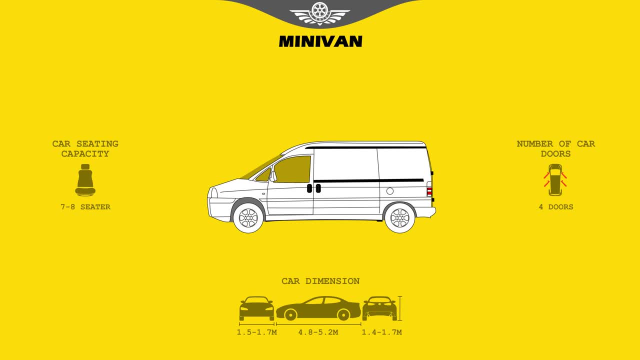 They're more of a cargo bay type of car. They have two boxes on wheels with sliding side doors for easy access and a rear hatch that opens to a large cargo area. Most minivans have adjustable seats in their second and third rows that often can be removed or even folded into the floor to create a 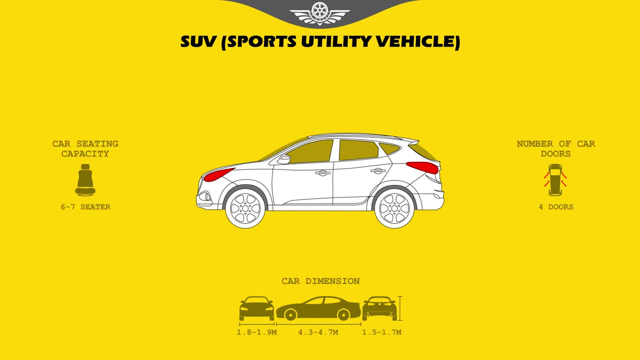 huge open cargo bay SUV. SUVs, often also referred to as crossovers, tend to be taller and boxier than a car. They include a station wagon-like cargo area that is accessed through a flip-up rear hatch door, and many offer all-wheel drive MPV. 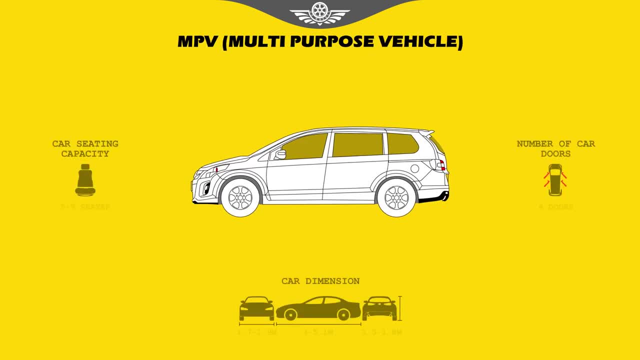 MPV, or multi-purpose vehicle as the name suggests, is made for playing various roles, But the most important of them all is transporting as much number of people. Five or seven-seater MPVs are considered to be a family vehicle, But they are mostly considered for commercial purposes, transferring tourist or office staff. 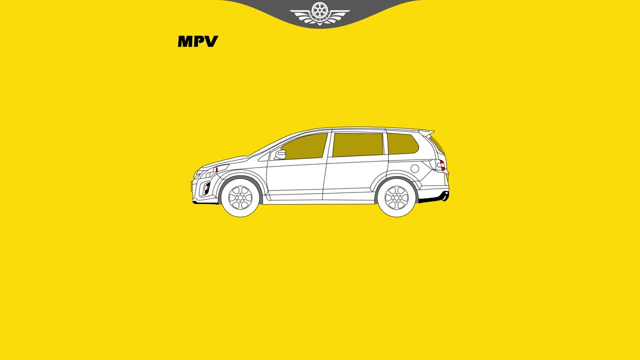 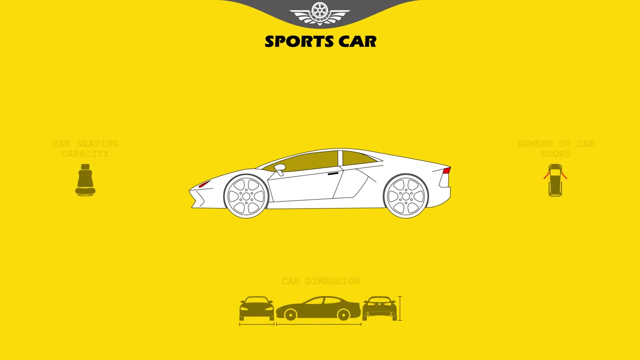 The reason is the low cost, fuel efficiency and passenger carrying capacity. Sports Car: These are the sportiest, hottest, coolest-looking coupes and convertibles: low to the ground, sleek and often expensive. They generally are two-seaters, but sometimes 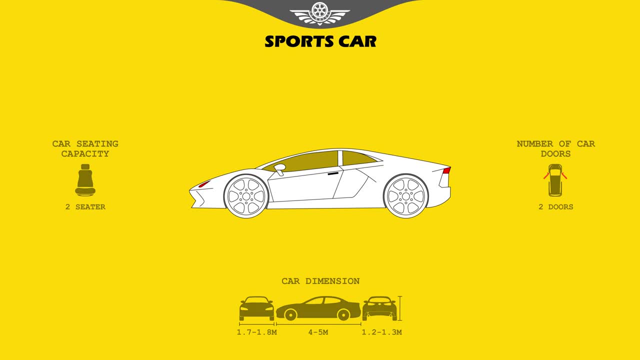 have small rear seats as well. There are the high-end exotic dream cars, which are also considered to be the most expensive cars with sky-high price. Pickup Truck: A pickup truck has a passenger cabin and open cargo bed in the rear- Virtually all. 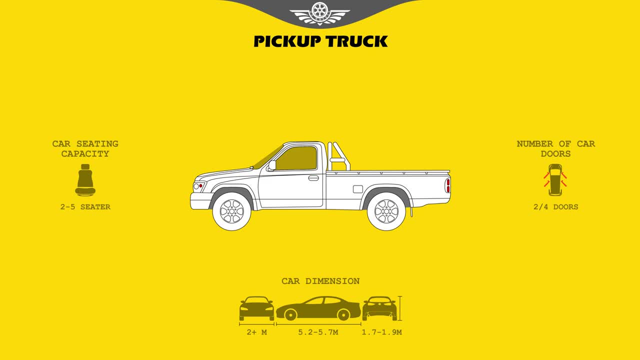 pickups offer some form of all-wheel drive or part-time four-wheel drive, the latter for off-road use only. Currently, pickup trucks come in two size categories: full-size and mid-size Station Wagon Wagons are similar to sedans but have an extended roofline and a hatch door at the. 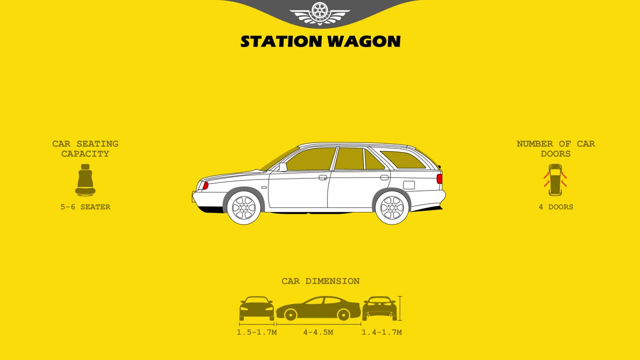 rear instead of a trunk. This means that the car can be used as an off-road vehicle or as an off-road vehicle. Some have elevated ground clearance and some rugged body cladding to make them more like a sport utility vehicle, but they are nonetheless closely related to sedans. 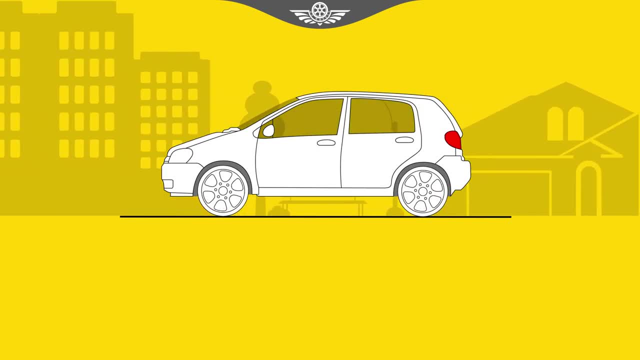 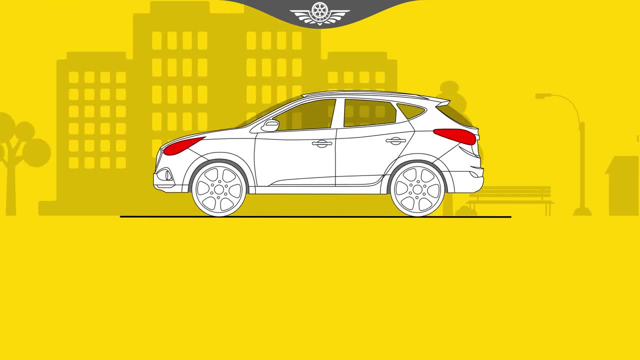 It doesn't stop there. There's more to it than basic body types. Those 10 types of vehicles are available from dozens of different brands and in many sizes and at widely varying prices. If you like the video, hit the like button, comment and subscribe to our channel for more videos. Thanks for watching.